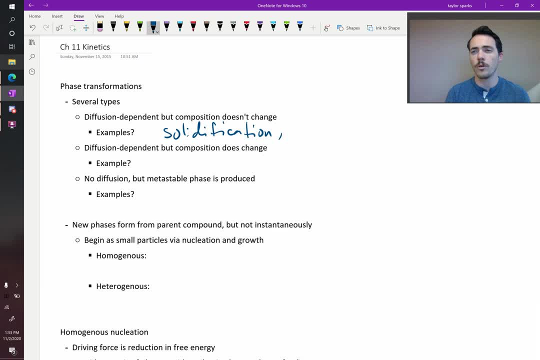 They have to diffuse and move into some sort of arrangement, but the overall arrangement doesn't change. Another example might be a change from one allotroph to another right. So diamond turning into graphite, for example, would be an example of a diffusion dependent transformation where there's no change in the composition. Now a second type of phase transformation is diffusion dependent but there is a change in the composition. Now we've seen lots of examples of this, For example the eutectic reaction right. 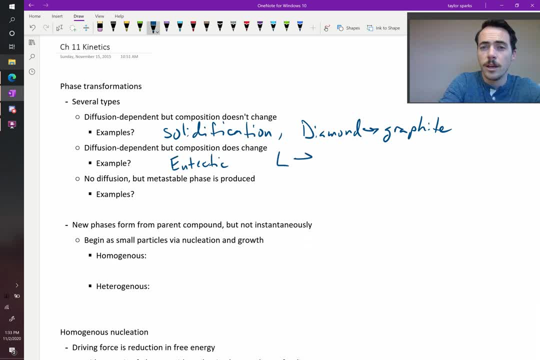 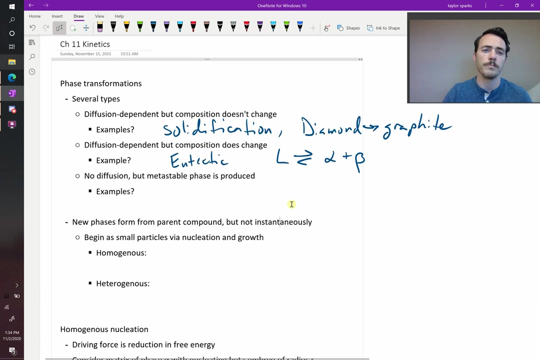 In a eutectic reaction, you start with a liquid at one composition and it splits into two solids at different compositions. right, So there has been a change in composition. Diffusion was present. okay. Now the third type says that there's no diffusion present, but it forms a metastable phase. We're going to give an example of this later on in this chapter when we talk about steel. There's a really important one Now. regardless of which type of phase transformation we're talking about, they all include these components. 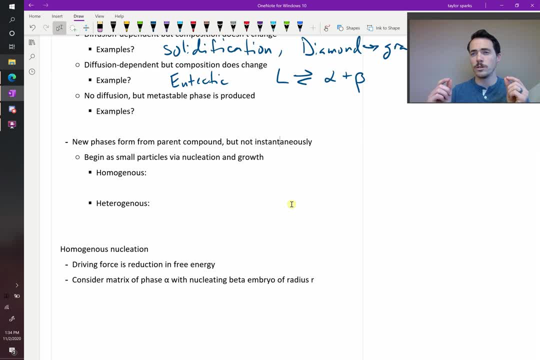 You start out with a parent phase, You're going to switch it to your new phase, and it doesn't happen instantaneously, right? This is not an instantaneous reaction. Instead, it starts out with a little nucleus. right, It starts out as a small particle. This nucleus can then either shrink and disappear or it can grow, right. So nucleation and growth. And when it comes to nucleation and growth, there's two different categories. You can have homogeneous nucleation or heterogeneous nucleation. So what's the difference? 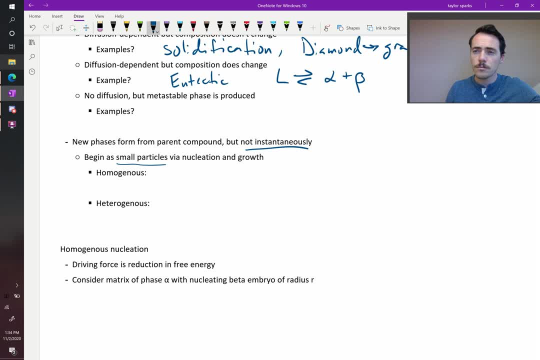 Homogeneous nucleation is one that takes place uniformly throughout the bulk of the material right. Now, in contrast, it can happen via heterogeneous nucleation And in that scenario it's going to happen at structural inhomogeneities in your material. These might be surfaces, insoluble particles, grain boundaries or dislocations right. 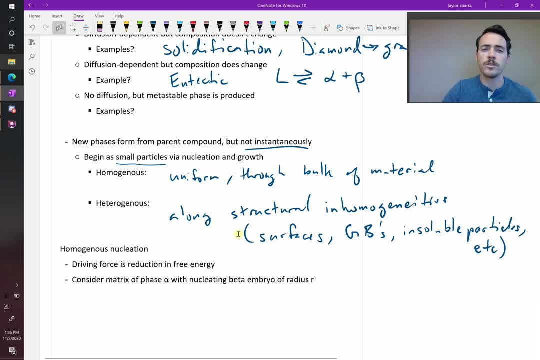 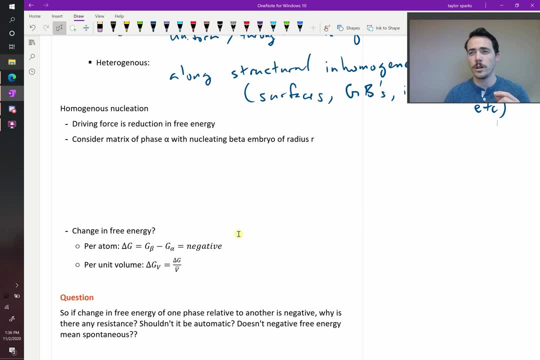 So let's first talk about homogeneous nucleation. All right, what's the driving force? Why does something happen? Why is it going to transform from one phase to another? We know why We talked about free energy already. It must be lowering the Gibbs free energy of the system, or rather the change in the Gibbs free energy right On a per atom basis. this change in Gibbs free energy must be going from a high energy to a low energy. right, And remember, in homogeneous nucleation it's happening in the bulk of material. So let's assume that we start out with, let's say, 100% liquid, right? So we'll call this the beta phase. It's a liquid. In homogeneous nucleation. you're going to form a little particle in the center of that right. This is an alpha particle. 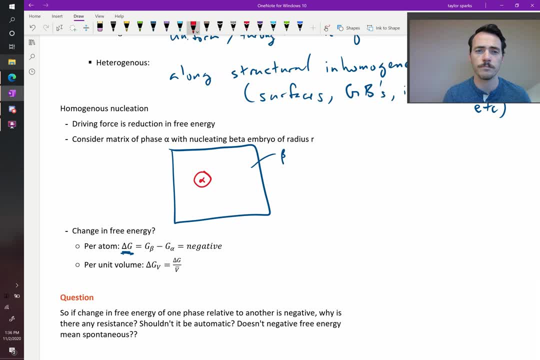 Some sort of solid, as it's solidifying from a melt. okay, Now what do we know about this? On a per atom basis, what is the change in Gibbs free energy? Well, the Gibbs free energy of these atoms in the beta phase. if we subtract from that the Gibbs free energy of those in the alpha phase, it has to be a negative number for this to be thermodynamically favorable. But we do this instead on a per volume basis. So we need to take the per atom basis and divide it by the molar volume, right, Because atoms can occupy different. 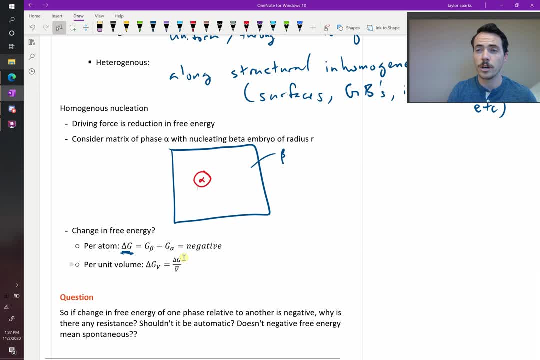 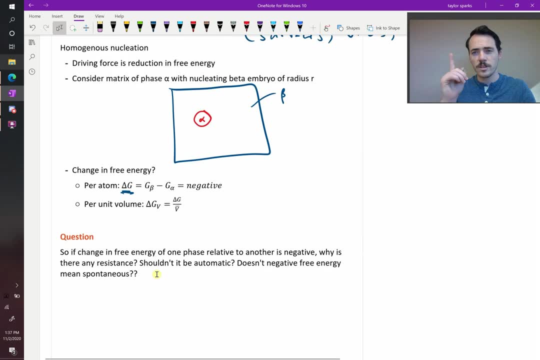 volumes. So if we take that change in the Gibbs free energy on a per atom basis, divide it by the molar volume, we now get this change in the Gibbs free energy on a volumetric basis. So the question is this: If the change in the Gibbs free energy on a volumetric basis is negative, right, So it's going down in energy to form this alpha particle, Why should there be any resistance, right? What possible reason could you have for there be a resistance? Shouldn't this just be automatic? Doesn't a negative free energy always mean that it's 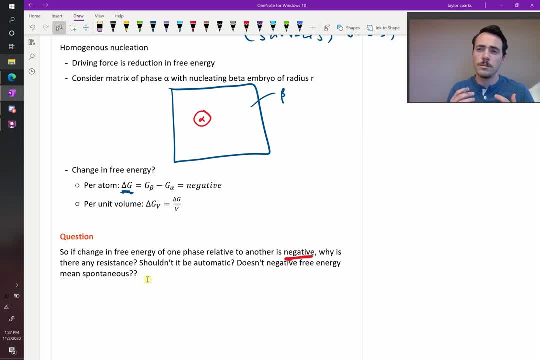 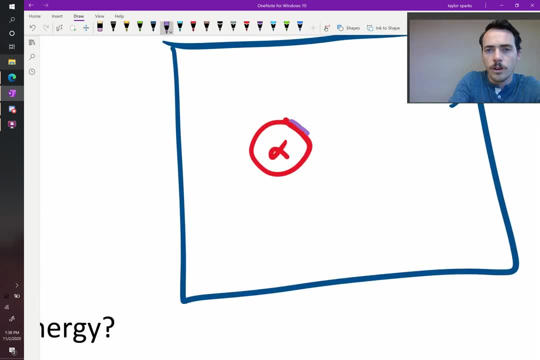 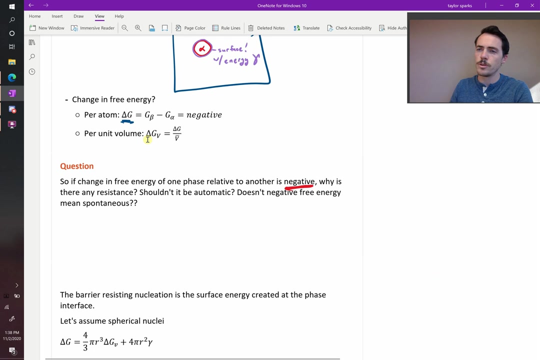 going to be spontaneous? Well, not necessarily. And how come? Well, think about it. At the interface of this particle, all along the interface of that alpha and the beta phase, what do you have? You have a surface, And a surface has a surface energy, right, We'll call that gamma. It has a surface energy, gamma, right? So no, it's not necessarily true that it's always going to be spontaneous, because surface energy is going to be a penalty as you form. 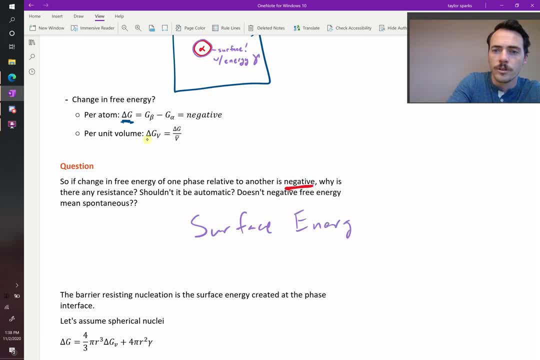 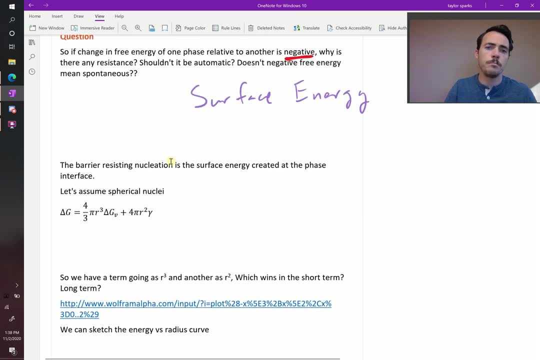 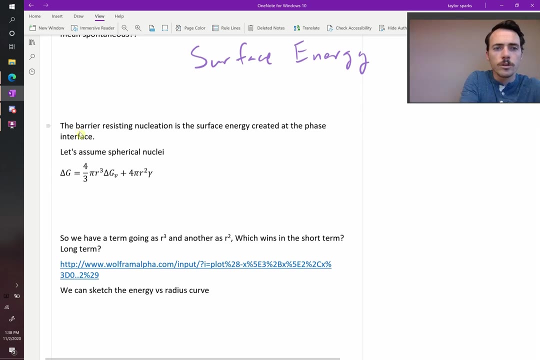 that new phase, you have to worry about surface energy potentially working in contradiction to your phase transformation. Therefore, this barrier needs to be calculated. Let's calculate the overall change in the Gibbs free energy right, Our overall change in the Gibbs free energy. take into account not only this component right here, the volumetric change in the Gibbs free energy, but let's also include this surface energy component. 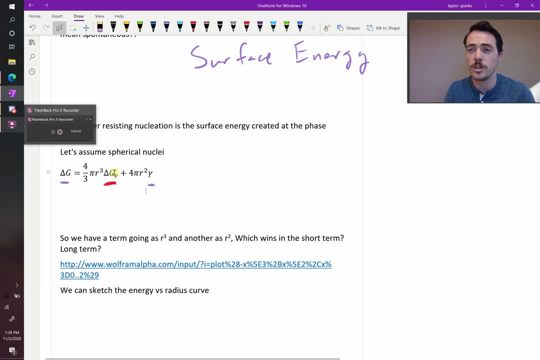 Now, in one case, since we're talking about changing the Gibbs free energy on a volumetric basis, we're going to need to include the volume of a sphere, And the volume of a sphere can be calculated as four thirds pi r cubed, where r is the radius of this new particle that's forming this new nucleus right, So it has some radius r. Meanwhile, the surface area of a sphere is four pi times r squared. So this is interesting. You have this competition where you've got two types of 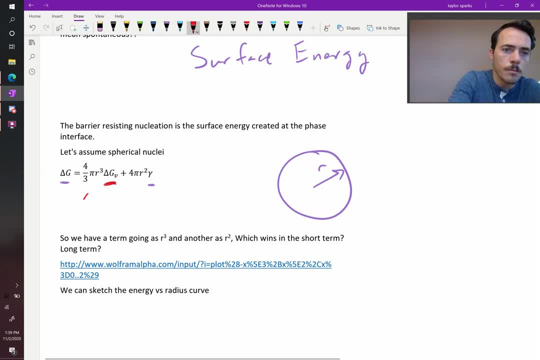 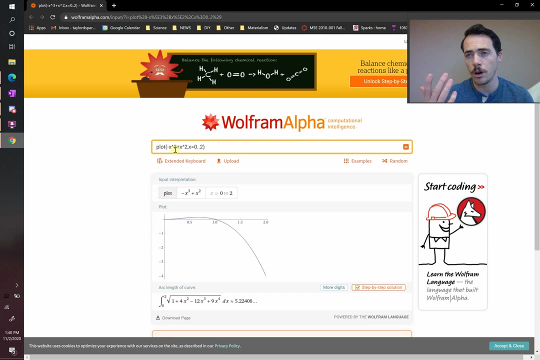 terms. This first term over here is negative And the second term over there is positive. So if you have a negative term multiplied by something by r cubed and a positive term multiplied by something to the r squared and you plot those both as a function of r, how does that function look? Let's take a look at Wolfram alpha and see. Well, you can see here I've plotted negative x cubed, so r cubed plus a positive x squared, right Gone, going from zero to two, and I've left off all the 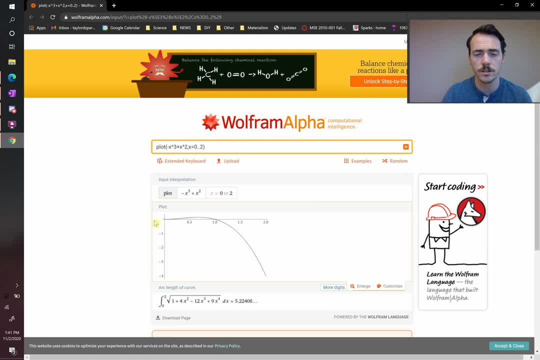 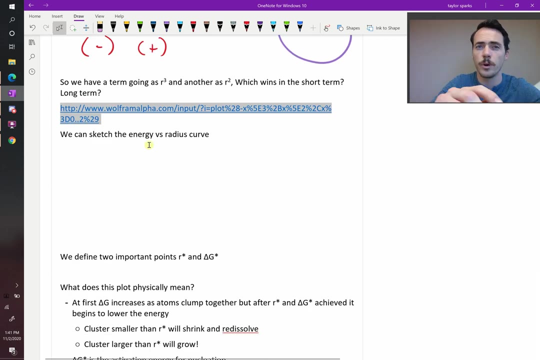 other coefficients, But still, you can see that the general expression looks like this: The plot rises at first and then it falls, right? So it's initially going to be a positive number and then it's going to be a negative one in this expression, right? So that allows us to sketch this change in energy as a function of the radius curve. So here's our radius of the new solid particle that's forming from the liquid phase. right? That's the size of our nucleus. Here is our energy. right, The change in the Gibbs free energy.